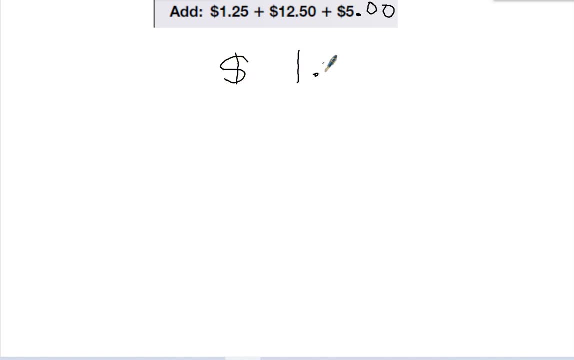 So I have $1.25 plus $12.50 plus $5. So decimal comes straight down. And then I add like I normally do. 5 plus zero plus zero is 5. 2 plus 5 is 7 decimal. 1 plus 2 is 7 decimal. 1 plus 2 is 2 and two is 6. sincere sense here. So I can literally pop this. 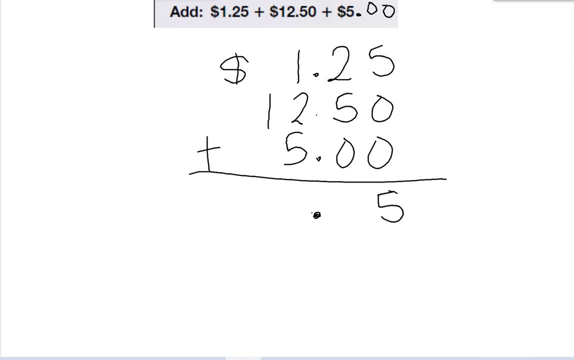 And plus my first and last digit there, thatимо, goes behind theしゃ. So this is where I don't need any addition. So I'm going to make sure that the middle digit comes out of my middle нажfer. And then I'm going to suddenly I'll copy this par. Square is when it comes to where I arrive, I have and this has to be square, correct? This is when it's an odd, let's say tidy on there. So I dry my entitled, and I wipe out my all, and then I give it to a square. I don't know if this create a new backhand and I need to add something to that exact addition. is 5, 2 plus 5 is 7, decimal, 1 plus 2 is 3, plus 5 is 8, and 1 plus nothing is 1. So 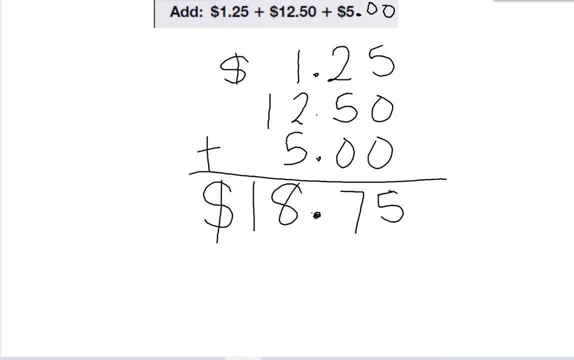 my answer is $18.75. Now when we subtract numbers, we also need to line up the decimal place or the place value. So we have 345 minus 67. Now in this case, I cannot take 7 away from 5, so I need to borrow from the next place value. I'm going to borrow from the 4, the 4 becomes a 3, and the 5 becomes a 15. So 15 minus 7 is 8. Now I cannot take 6 away from 3. 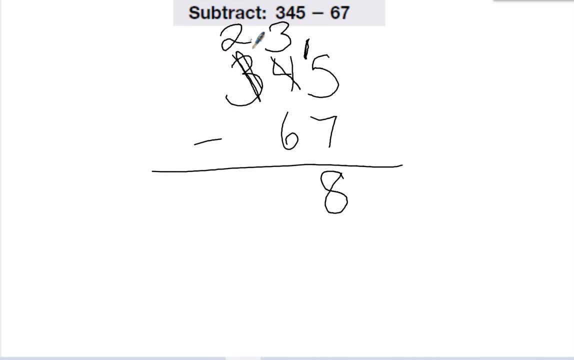 So I need to borrow again. This 3 becomes a 2, and the 3 becomes a 13. 13 minus 6 is 7, and 2 minus nothing is 2. So my answer is 278. 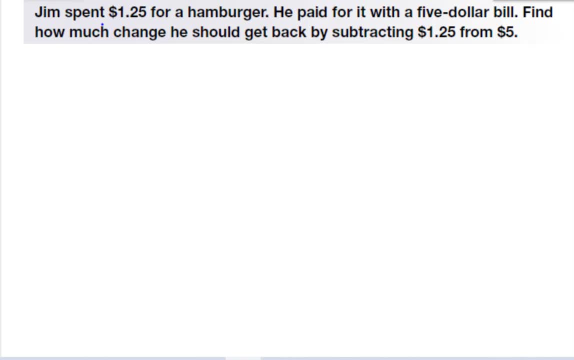 So here I've got a word problem. It says Jim spent $1.25 for a hamburger. He paid for it with a $5 bill. Find out how much change he should get back by subtracting $1.25 from $5. 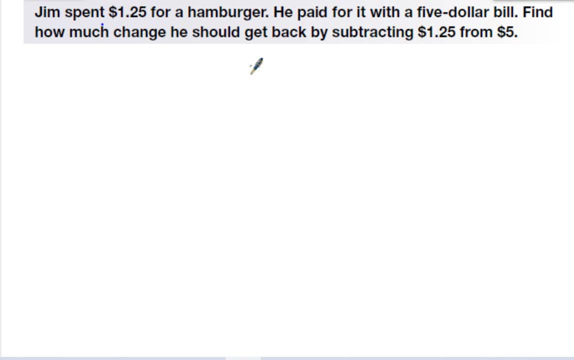 So just like before, I need to take this $5, and I need to give it a decimal point and some 0s. That way I can line up the decimal points in $1.25. And just like when we always subtract, we have to borrow. So I need to come all the way over to the 5. 5 becomes a 4. This 0 becomes a 10, which I need to borrow from that to make this 0 a 10. 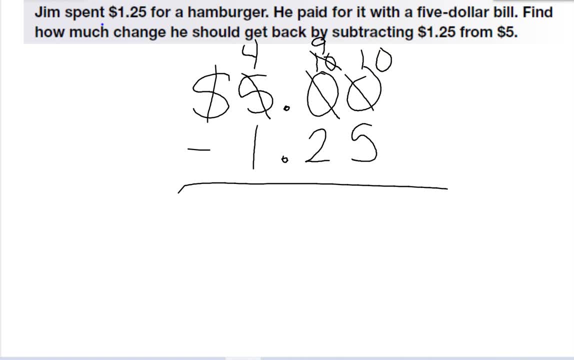 So I need to come all the way over to the 5. 5 becomes a 4. This 0 becomes a 10, which I need to borrow from that to make this 0 a 10. Also I can add that $5 into $1 to make this 0 . So 10 minus 5 is 5, 9 minus 2 is 7, decimal place, 4 minus 1 it 3. So he should get back three dollars and 75 cents after paying for his hamburger. decimal place for minus one is three so he should get back three dollars and 75 cents after paying for his hamburger. 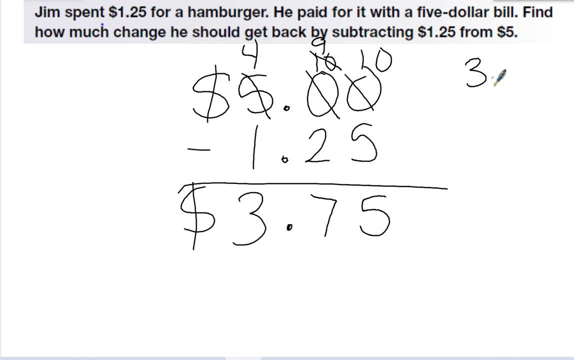 Now if you want to check, you can always take three dollars and 75 cents and add $1.25. 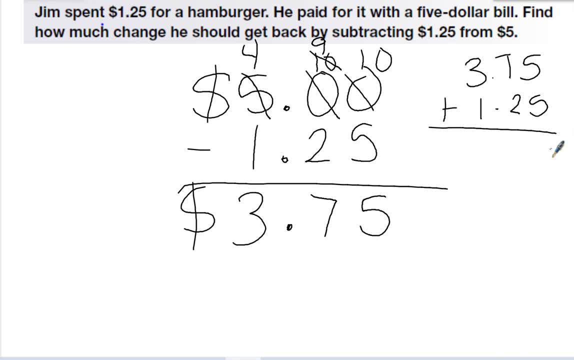 If our answer is correct we should get $5. So 5 plus 5 is 10, 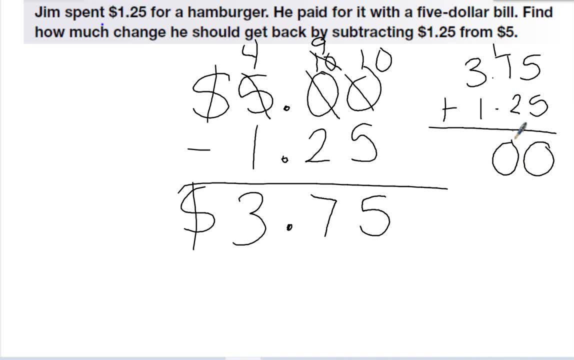 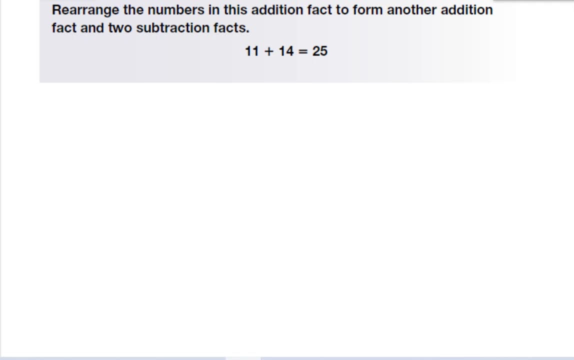 the 1. 1 plus 7 is 8. Plus 2 is 10. Carry the 1. Decim point down. 3 plus 1 plus 1 is 5. So my answer is correct. All right, so now we need to do some fact families. Fact families are how we show 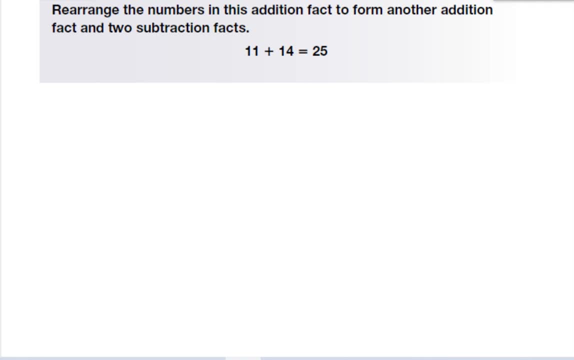 the different numbers and how they relate to each other. So this says rearrange the numbers in this addition fact to form another addition fact and two subtraction facts. So here I have 11 plus 14 equals 25. Now we know that we can also do 14 plus 11 equals 25. Okay, and then my two subtraction facts are always going to be the biggest number here. So 25 minus the other number 11 equals 14 and 25 minus 14 equals 11. When we do fact families, we can only use the three numbers 11 and 14. So we can only use the three numbers 11 and 14. So we can only use the three numbers 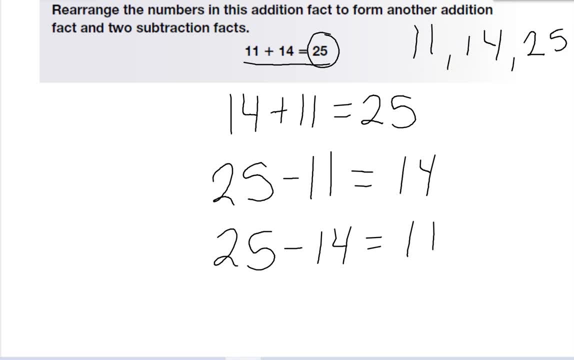 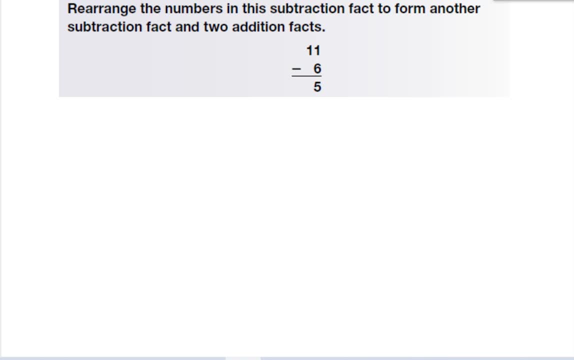 11, 14, and 25. Okay, so this is rearrange the numbers in this subtraction fact to form another subtraction fact and two addition facts. So we have 11 minus 6 equals 5. So the three numbers I can use are 11, 6, and 5. So let's do another subtraction. So I already had 11 minus 6. That means the next one is 11 minus 5 equals 6.